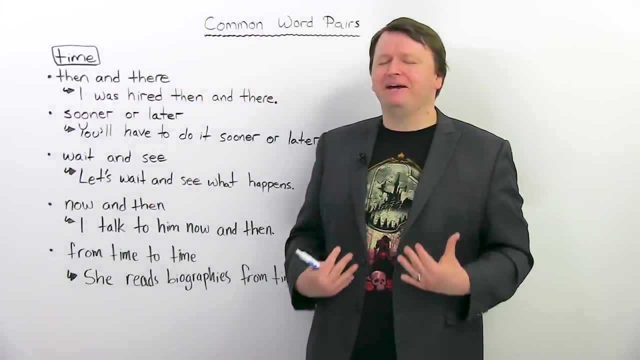 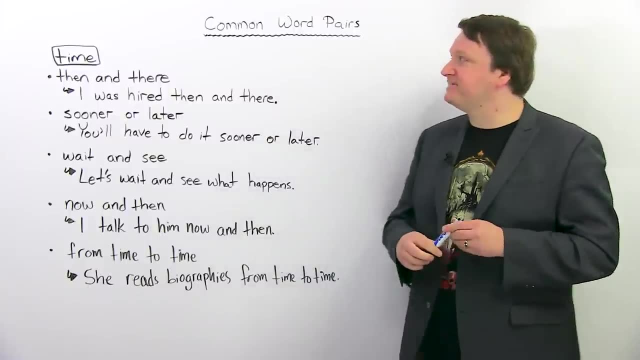 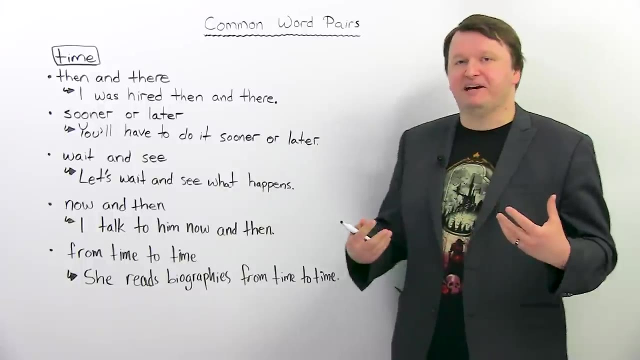 If you're lost, you can look and you will find me time after time. Hey everyone, I'm Alex, Thanks for clicking and welcome to this lesson on some common word pairs or expressions with time. So not just the word time, but different expressions. 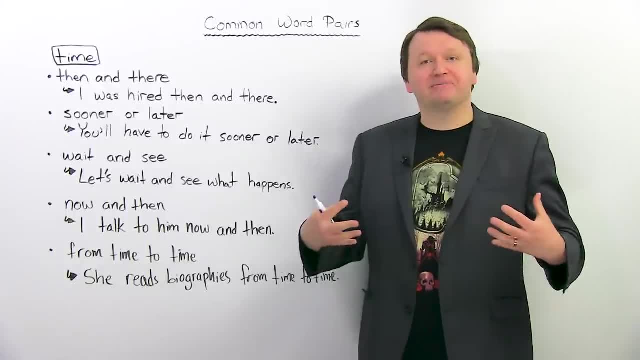 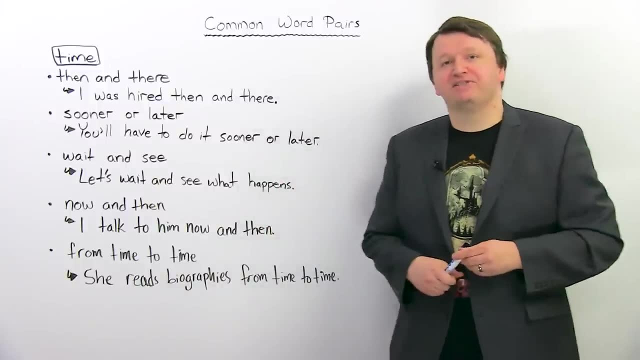 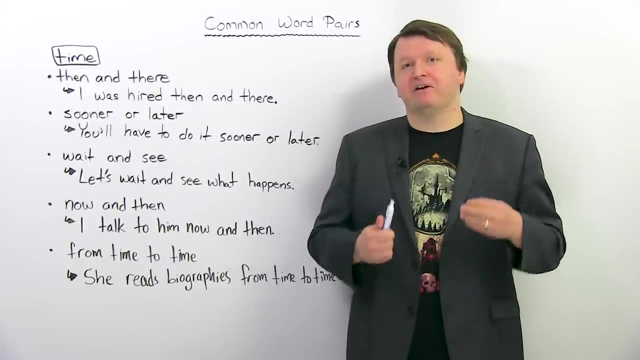 we use to indicate time or different expressions or word pairs. we use to talk about how long something takes or when something happens. So first we're going to look at five and then we're going to look at another five, and each time we go over one of these word 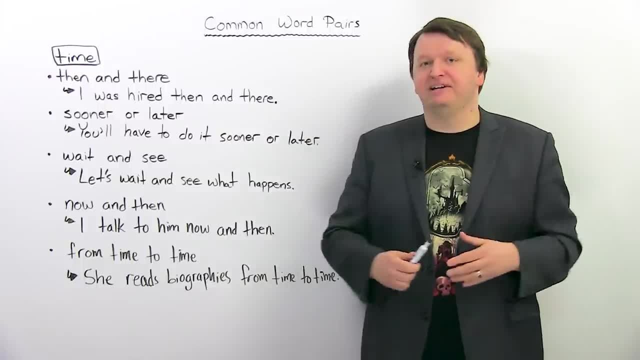 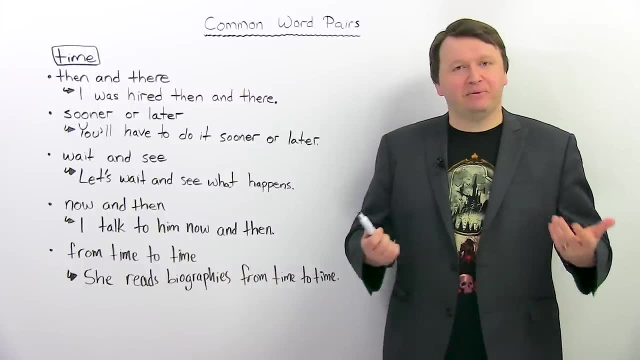 pairs. I'll give you an example sentence and I want you to you know. see if you can guess the meaning of this expression from the context, and then I will tell you the actual definition of you know what this expression or this word, pair, means. So let's. 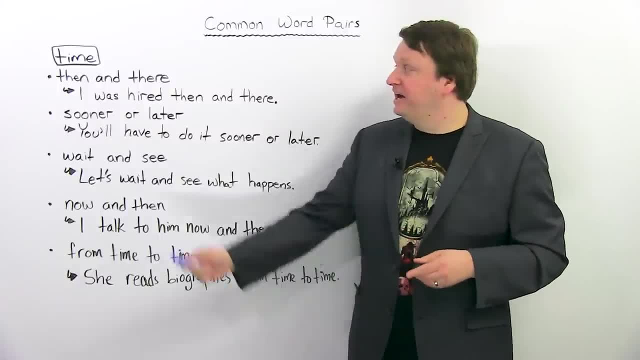 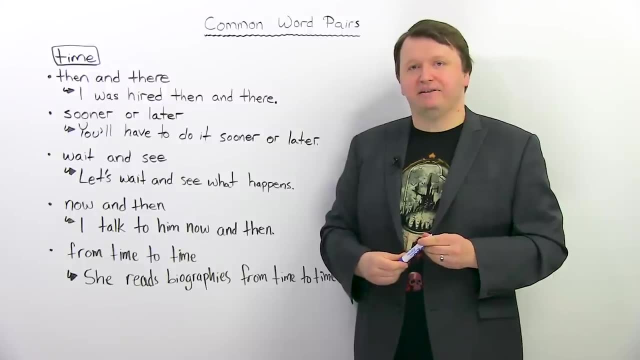 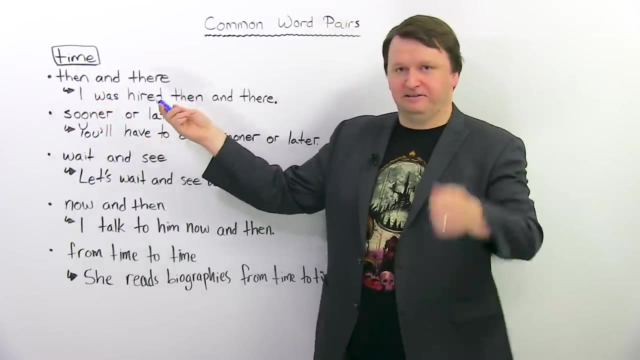 not waste any time, No more time. and let's begin Number one. then and there The sentence is: I was hired then and there Now, if you know the meaning, obviously, of then, at that time and there. 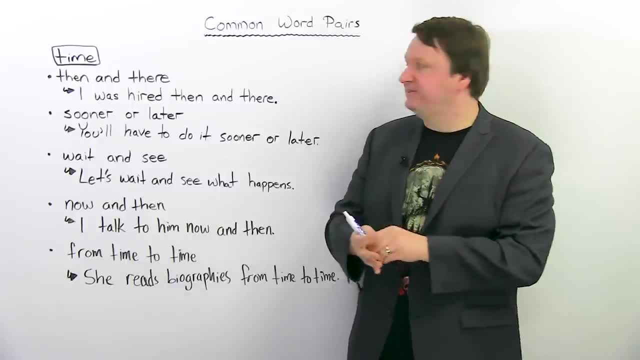 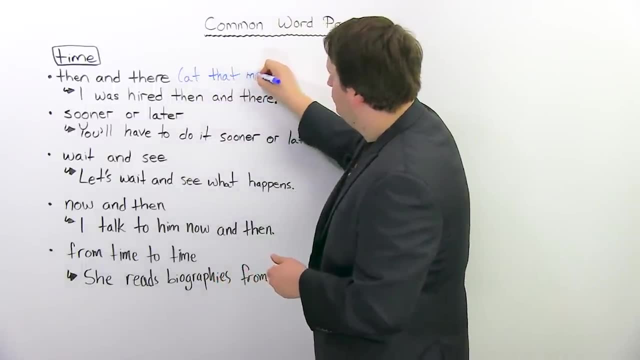 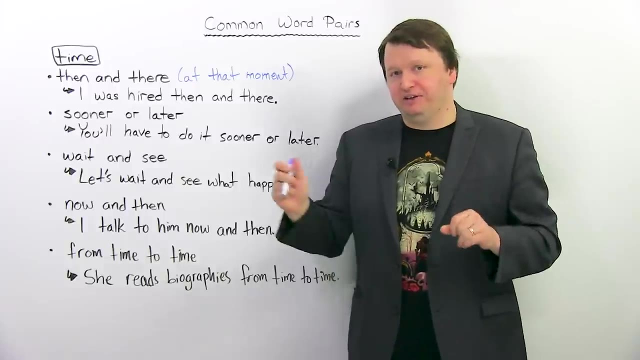 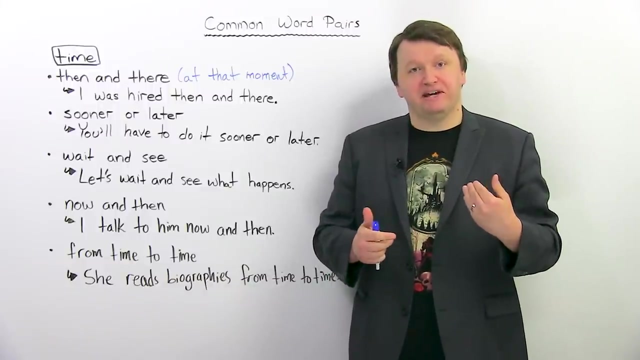 in that place. it means at that moment. Okay, So at that exact moment, At that moment. So imagine you go to a job interview in this case, and the interview goes very well. Sometimes the person who does your job interview says: okay, we'll call you back and we'll let. 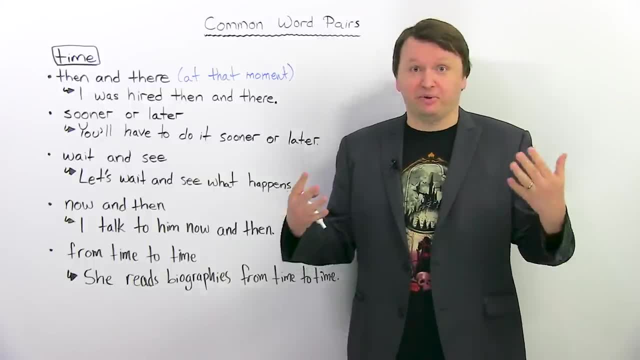 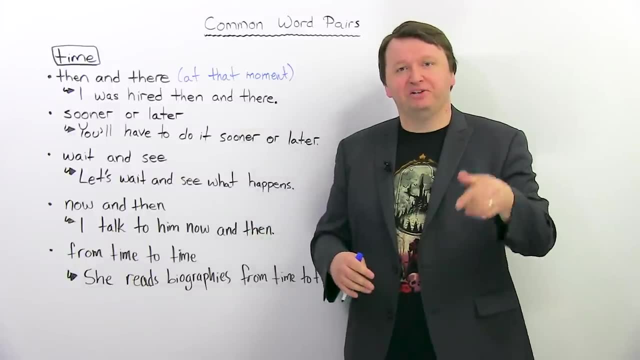 you know. but sometimes, if they know that you're the right person for the job, they will tell you when. they will ask you actually, when can you start, and they will hire you on the spot. They will hire you then and there, in that moment. 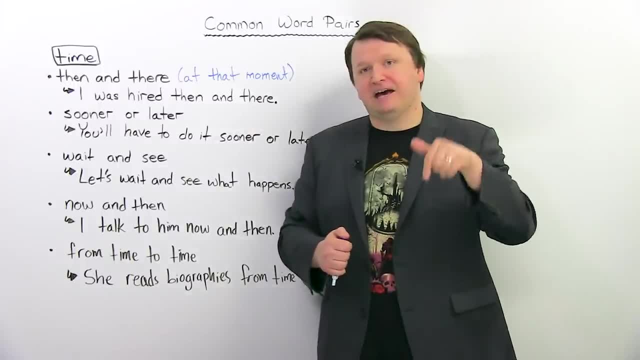 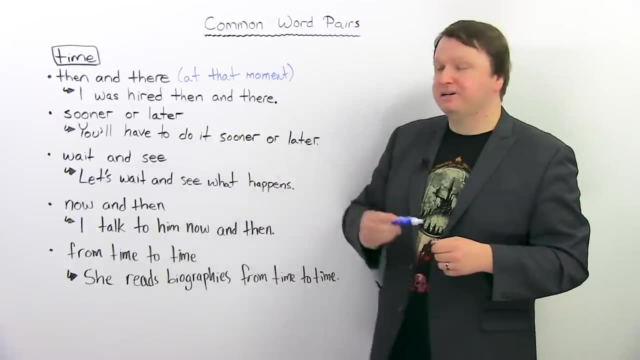 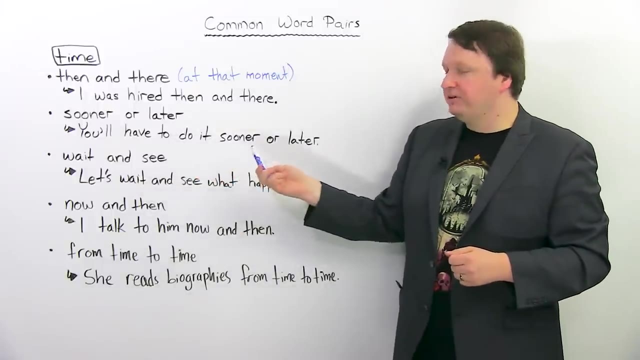 Okay. So that's what then? and there means at that moment. or she kissed me then and there I was hired, then and there Next. sooner or later, Sooner or later, You'll have to do it, sooner or later. 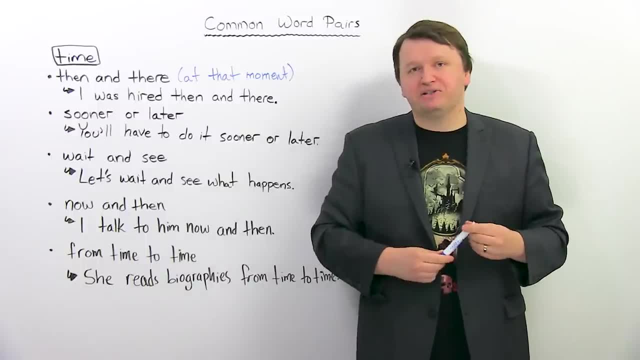 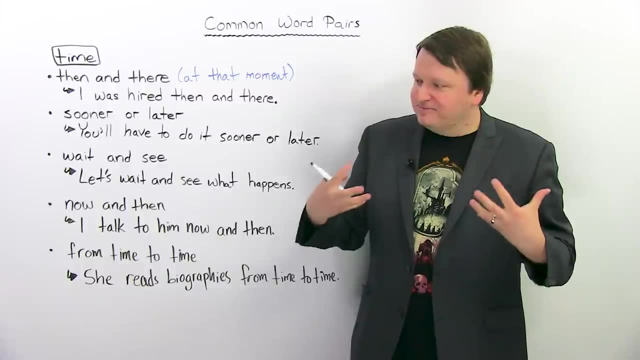 So most of us, I think, don't like washing dishes or we don't like doing the laundry and we just look at it in the corner. you know, telling ourselves: okay, we will do it, not now, later, later. 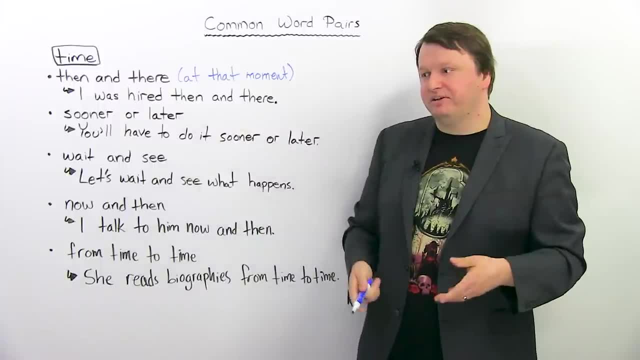 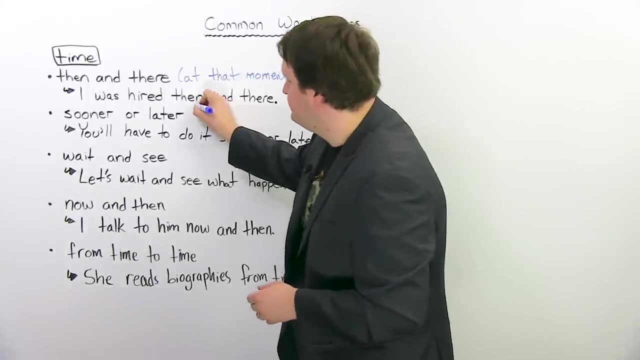 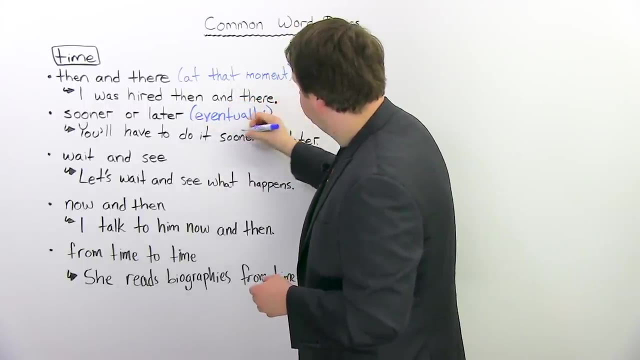 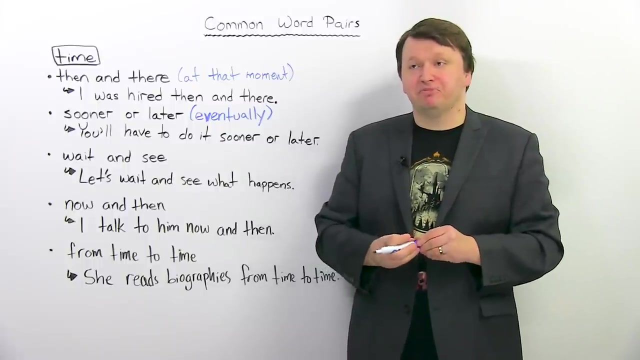 Okay, And maybe you know somebody will tell you: okay, can you do it now? because you will have to do it sooner or later, and in this case it means eventually. Okay, So sooner or later, So to say something a little more serious, sooner or later we're all going to die. 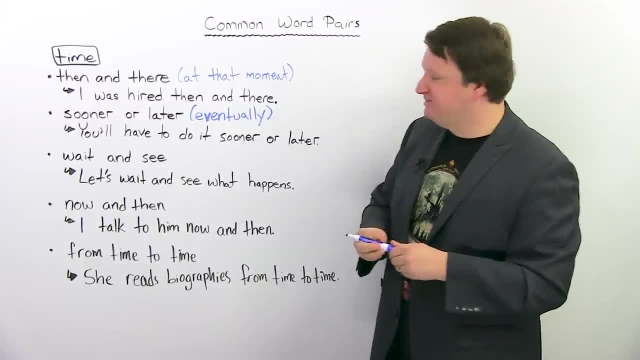 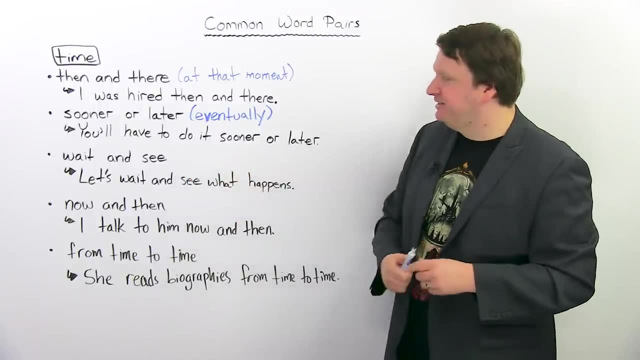 You know it's going to happen. It's going to happen. That's not the happiest memory or the happiest image, but you know, I think you get the meaning Sooner or later. Wait and see. Very simply. let's wait and see what happens. 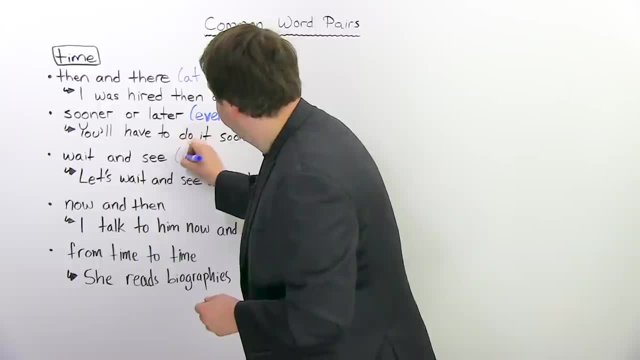 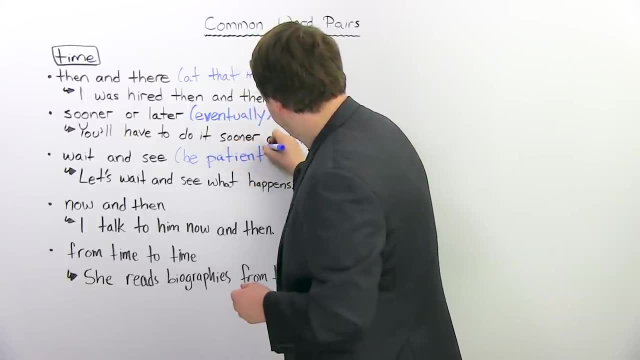 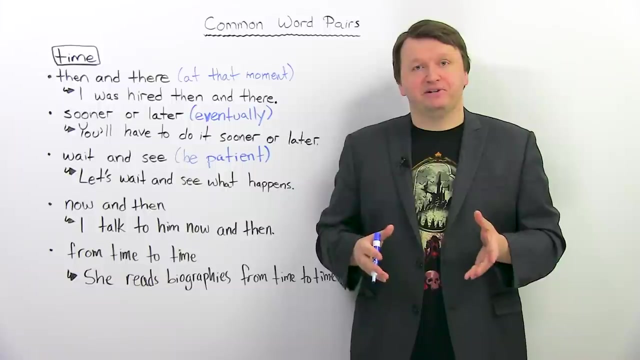 This just means: let's be patient, Be patient, Okay. So if you are watching a movie with a friend and your friend wants to know what happens next in the movie, because you have seen the movie before, and your friend's like, oh what? 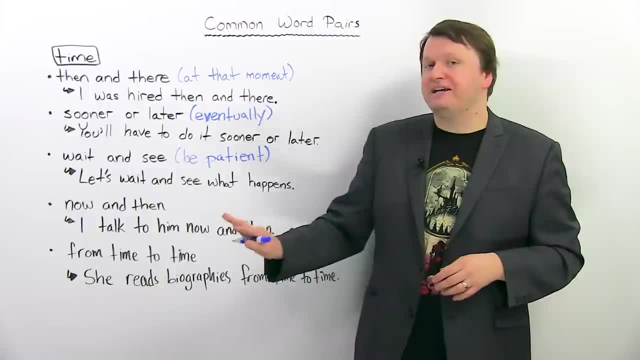 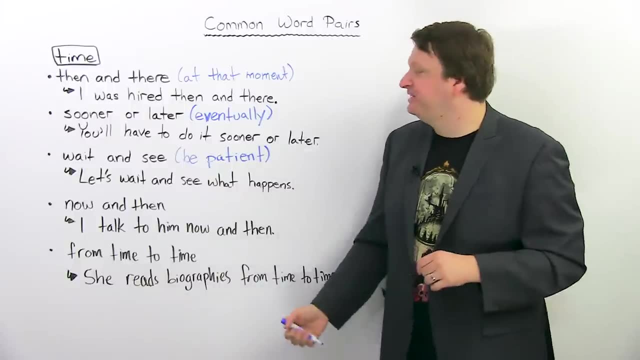 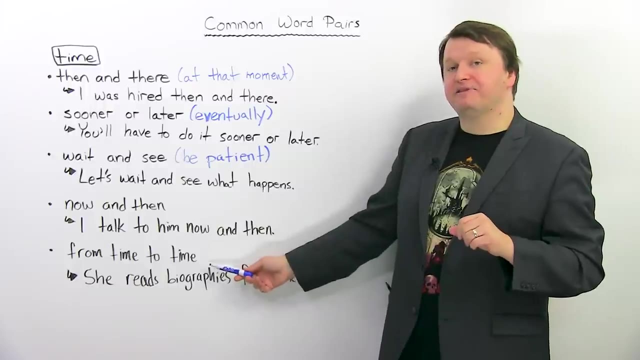 happens next? What happens next? And you just say wait and see And just wait and you will see what happens next. So just be patient. Now the final, The final two on the first board are very similar now and then from time to time. 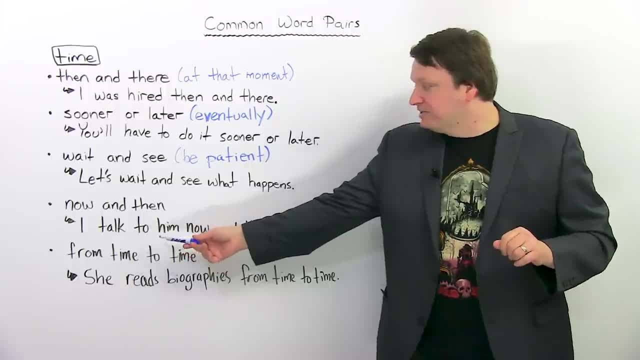 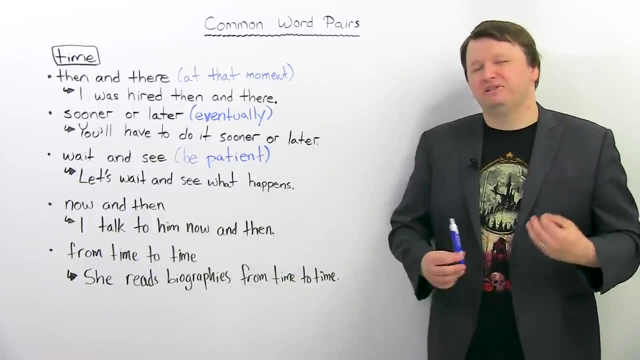 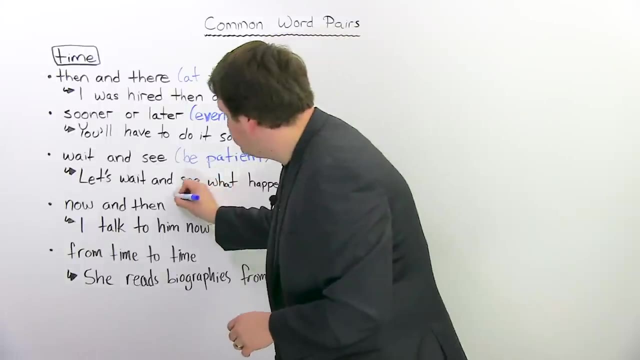 Both of these, if you look at the sentences. I talk to him now and then She reads biographies from time to time. What do you think these expressions mean? Sometimes, That's right. So infrequently, or sometimes Sometimes. 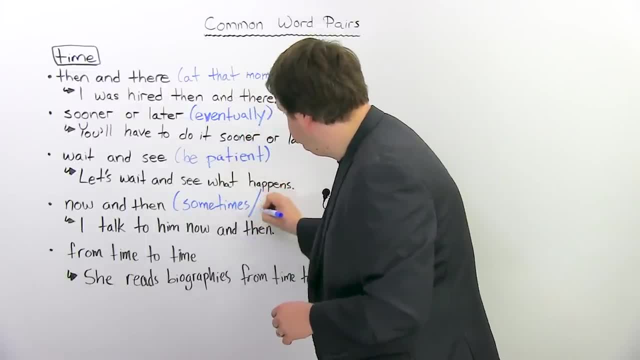 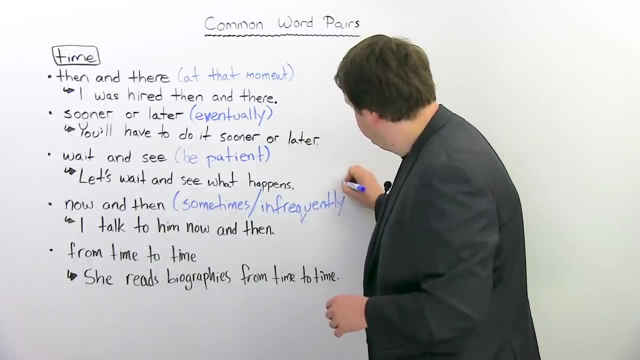 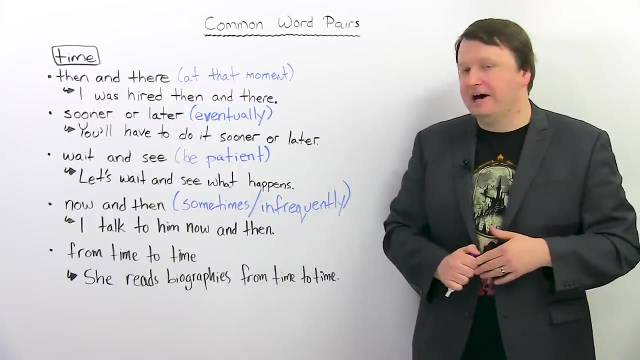 Sometimes. Another word maybe might be new for some of you guys: infrequently, not frequently, And these are interchangeable. Okay, So now and then. from time to time We go to restaurants. from time to time We go to restaurants, now and then.